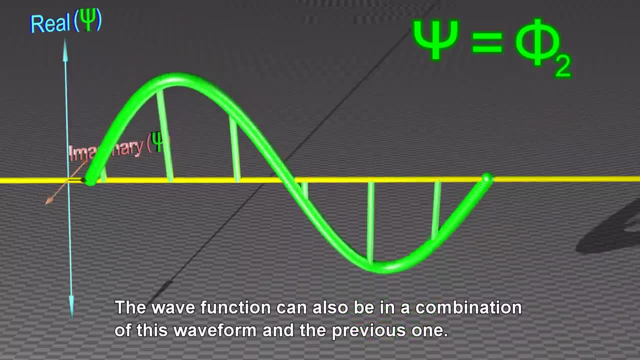 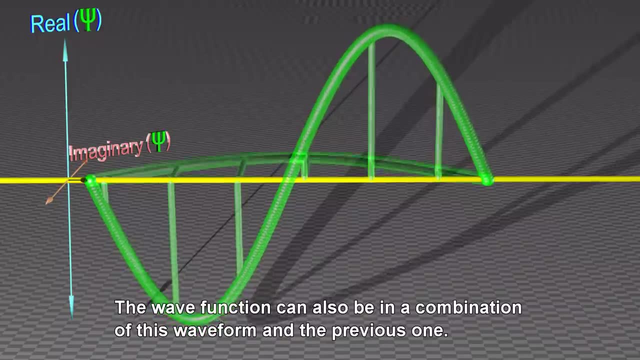 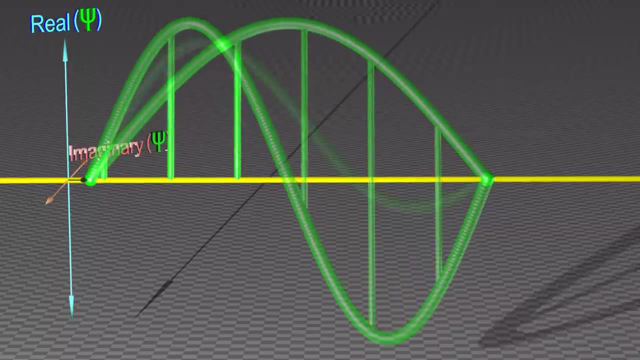 The wave function can also be in a combination of this waveform and the previous one. The wave function can also be in a combination of this waveform and the previous one. It may be in a combination of a wave function and a natural constant. For the next two simulations, the first one will be a wave function. 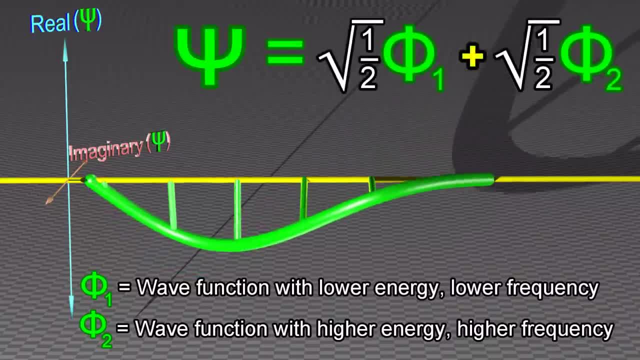 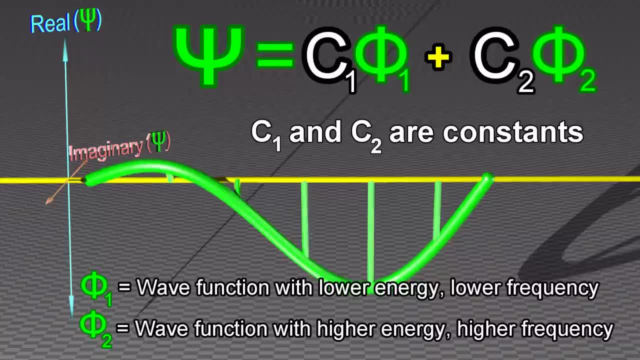 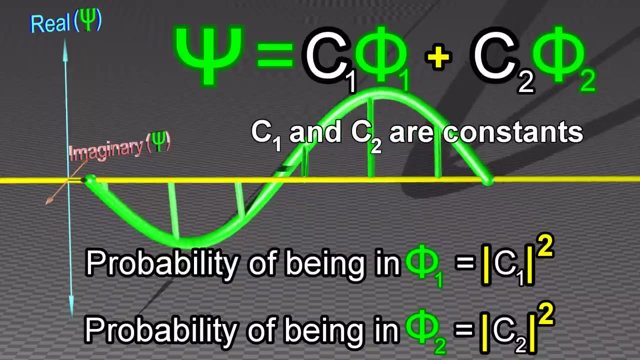 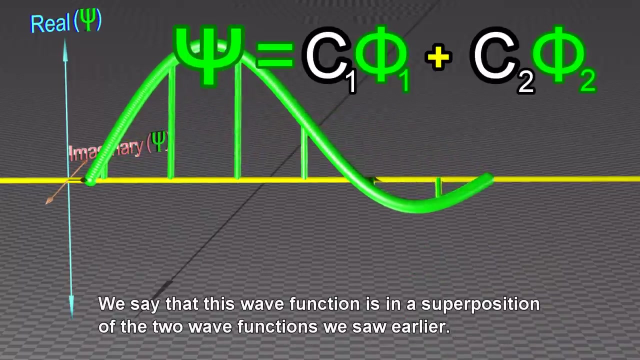 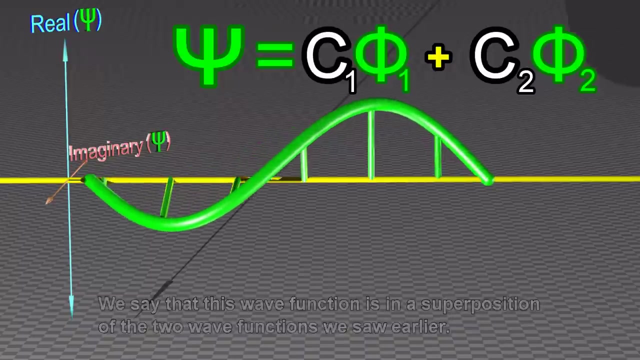 It can be in a combination of the two. The second time it will be a positive wave function. The third time it will be a positive wave function. We say that this wave function is in a superposition of the two wave functions we saw earlier. 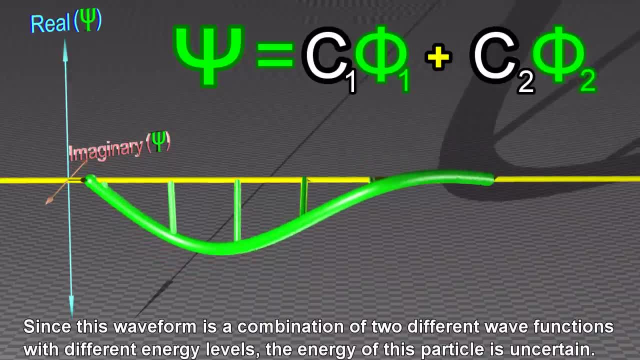 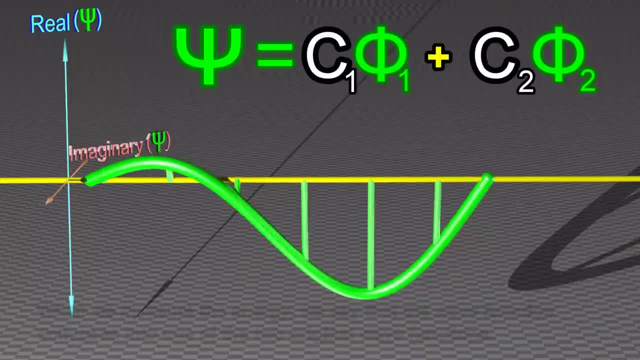 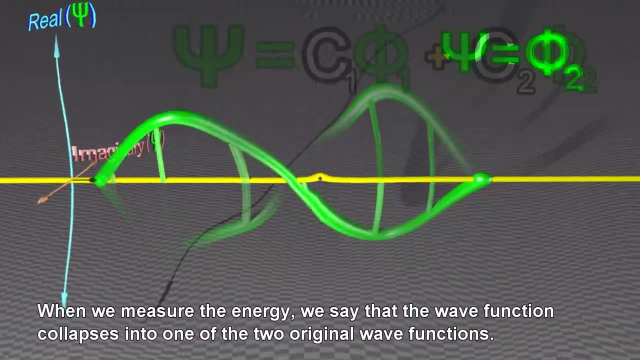 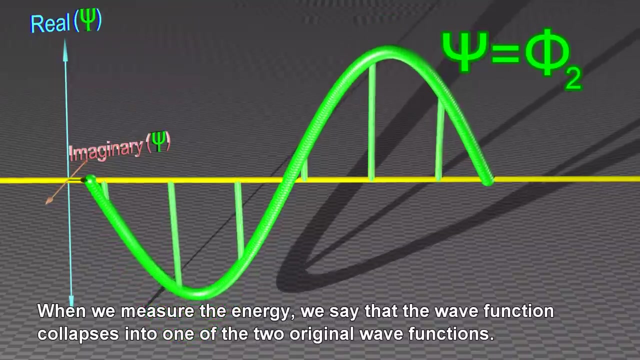 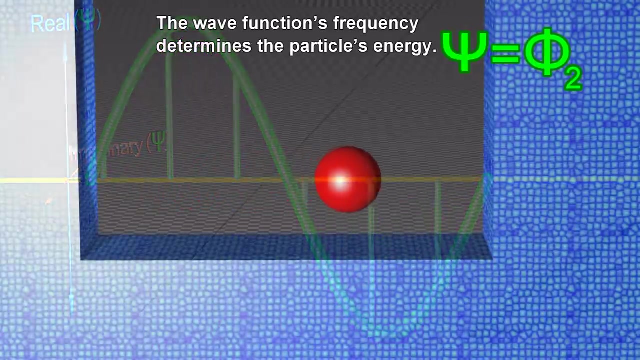 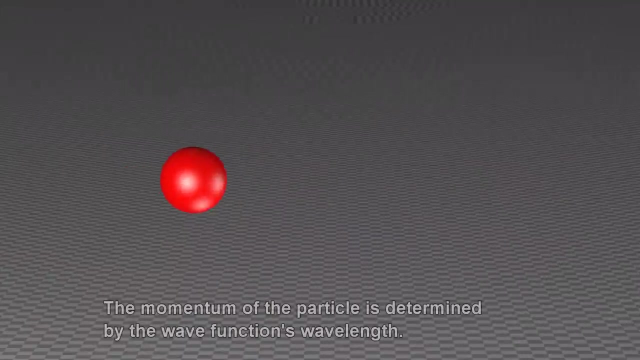 Since this waveform is a combination of two different wave functions with different energy levels, the energy of this particle is uncertain. When we measure the energy, we say that the wave function collapses into one of the two original wave functions. The wave function's frequency determines the particle's energy. 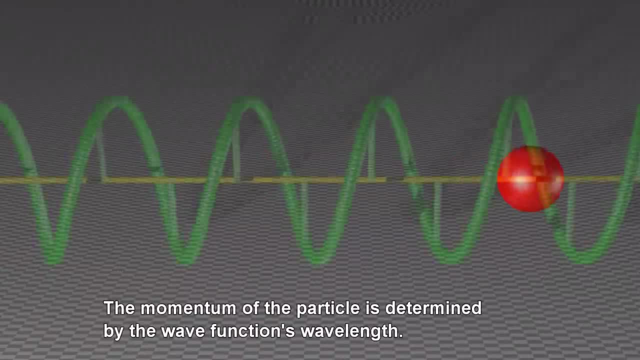 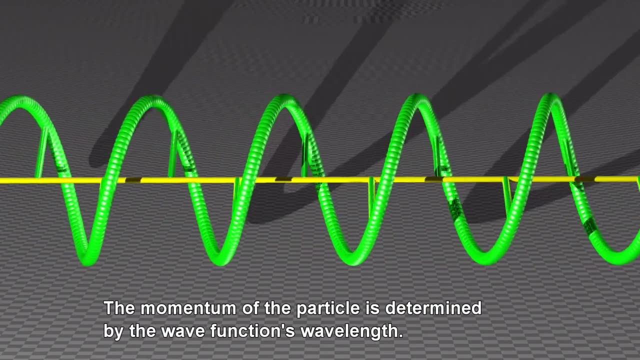 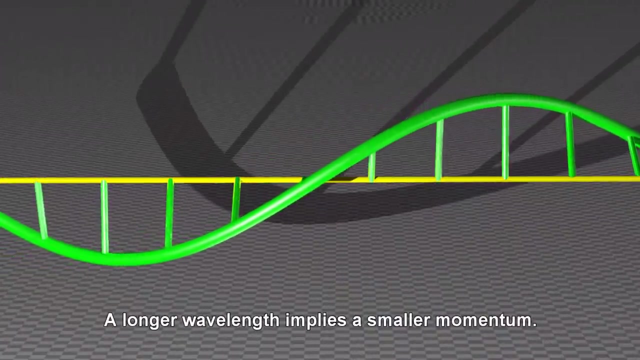 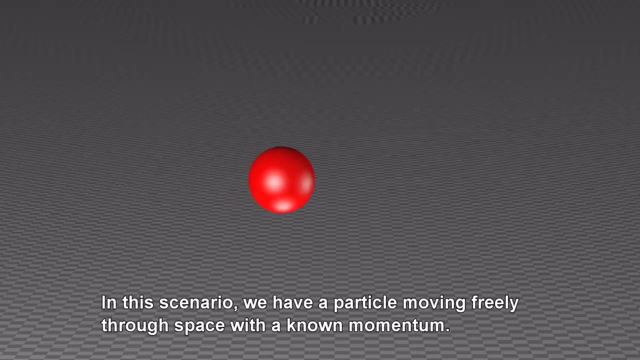 The momentum of the particle is determined by the wave function's frequency. The momentum of the particle is determined by the wave function's wavelength. A longer wavelength implies a smaller momentum. In this scenario, we have a particle moving freely through space with a known momentum. 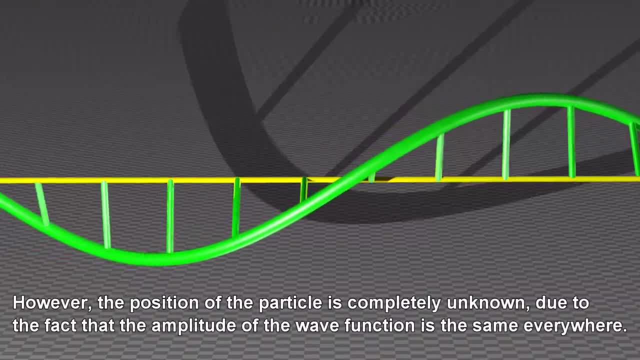 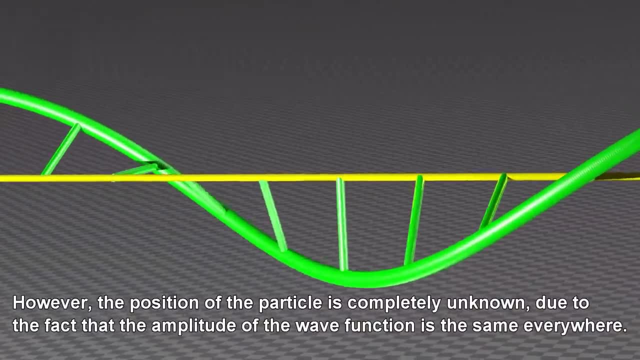 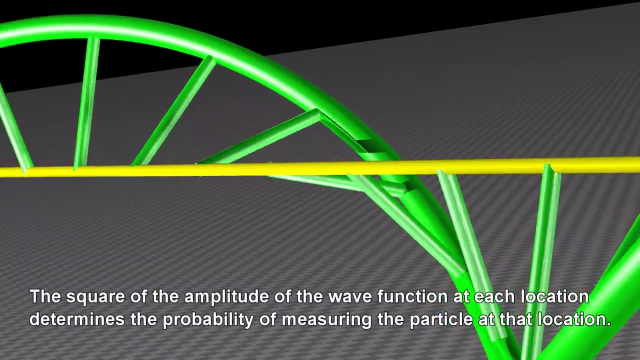 In this scenario, we have a particle moving freely through space with a known momentum. However, the position of the particle is completely unknown because the amplitude of the wave function is the same everywhere. The amplitude of the wave function is the same everywhere. The square of the amplitude of the wave function at each location determines the probability. 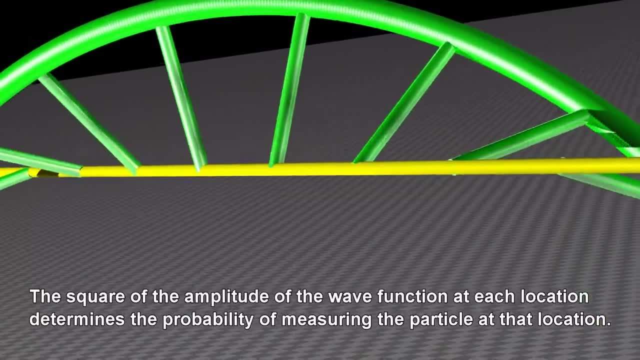 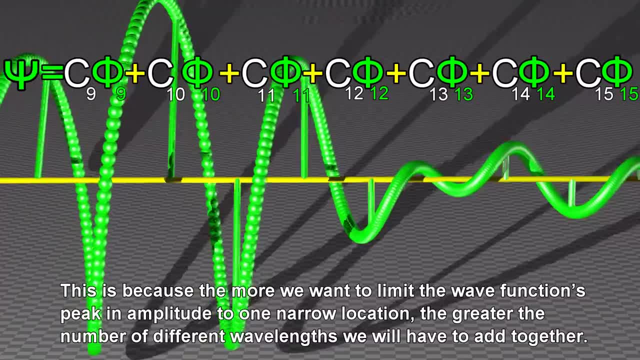 The square of the amplitude of the wave function at each location determines the probability of measuring the particle at that location. The square of the amplitude of the wave function at each location determines the probability of measuring the particle at that location. lengths we'll have to add together. 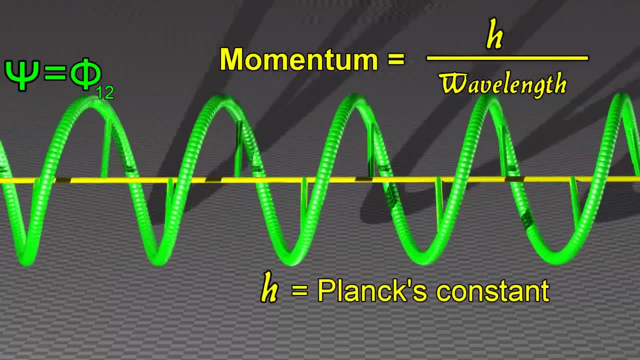 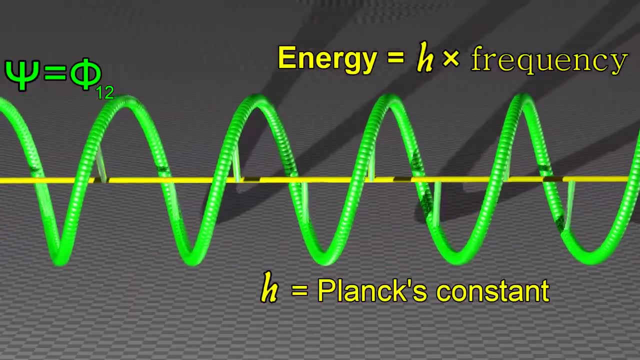 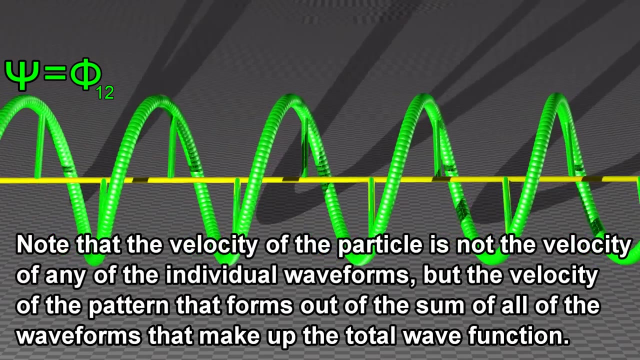 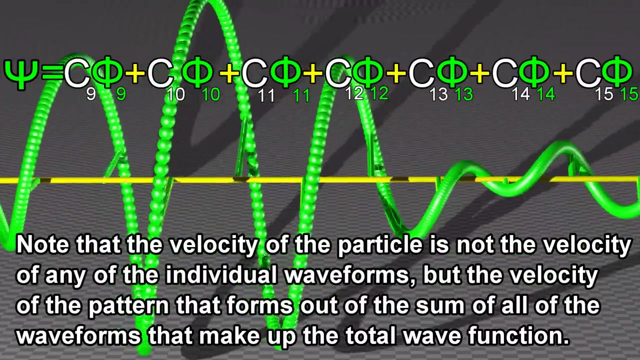 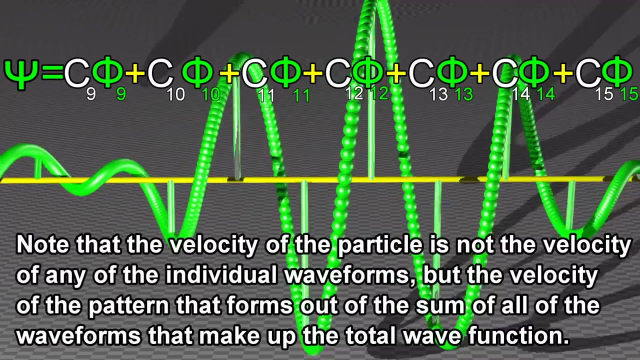 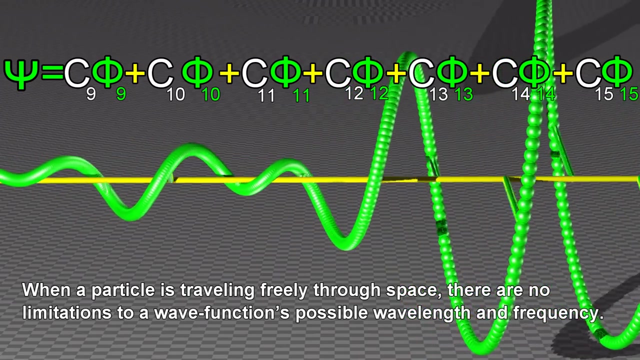 Note that the velocity of the particle is not the velocity of any of the individual waveforms, but the velocity of the pattern that forms out of the sum of all of the waveforms that make up the total wavefunction. When a particle is traveling freely through space, there are no limitations to a wavefunction's 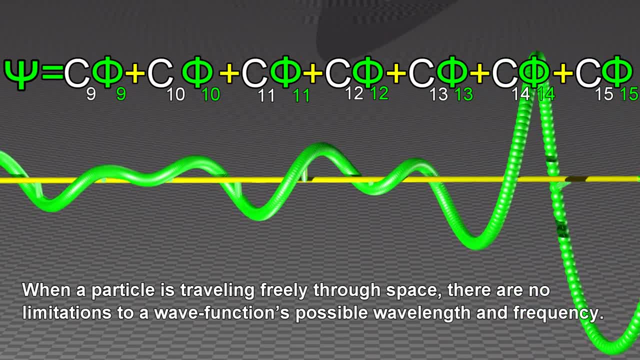 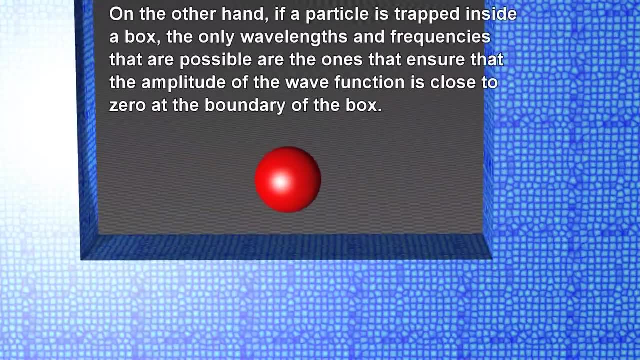 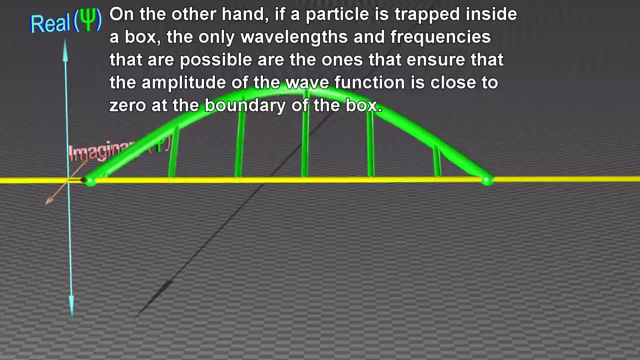 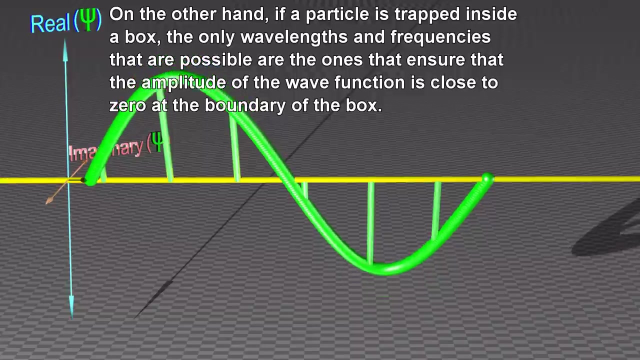 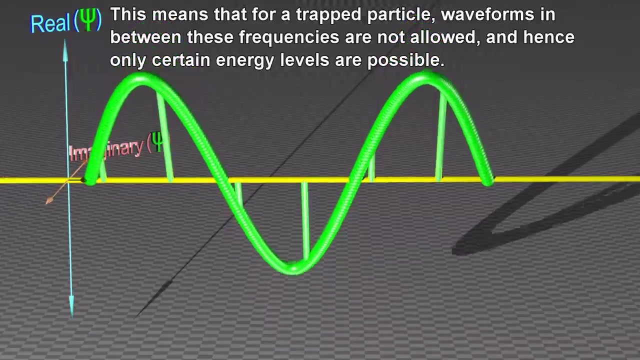 possible wavelength and frequency. On the other hand, if a particle is trapped inside a box, the only wavelengths and frequencies that are possible are the ones that ensure that the amplitude of the wavefunction is close to zero at the boundary of the box. This means that for a trapped particle, waveforms in between these frequencies are not allowed. 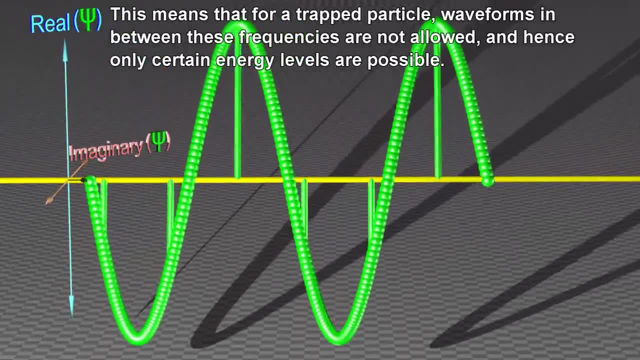 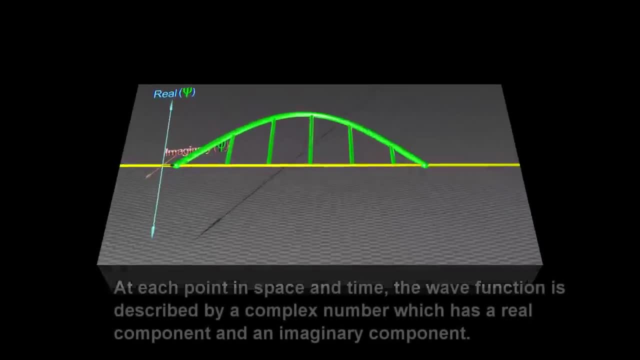 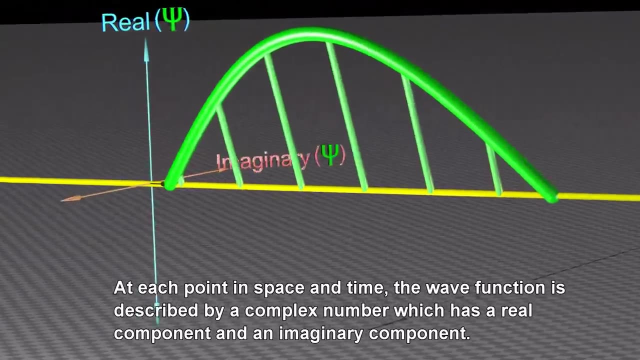 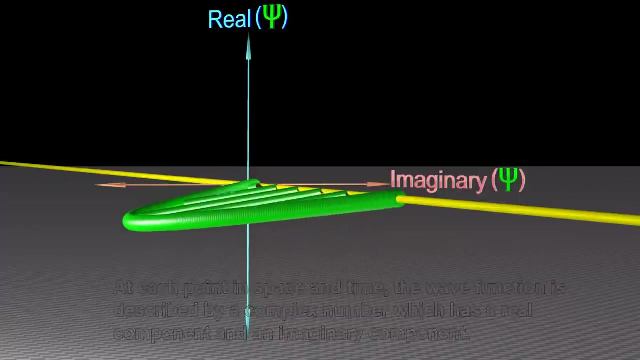 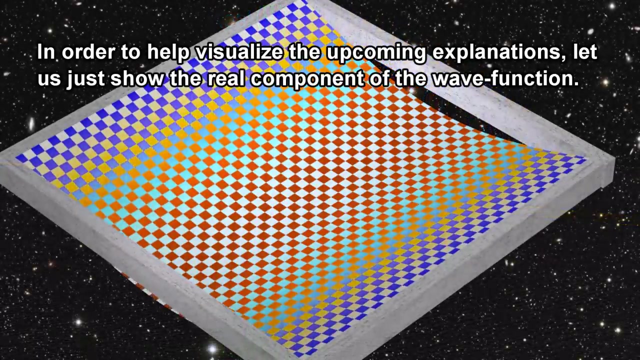 and hence only certain energy levels are possible At each point in space and time. the wavefunction is described by a complex number which has a real component and an imaginary component. In order to help visualize the upcoming explanations, let's just show the real component of the wavefunction. 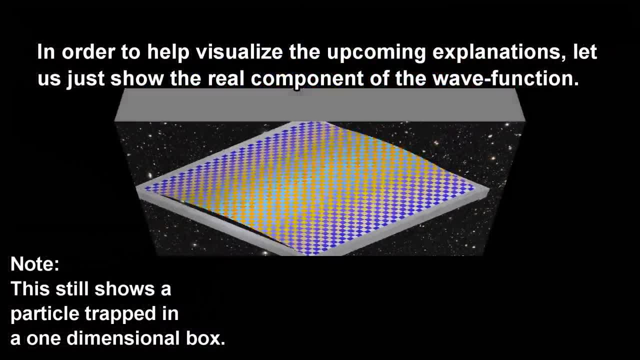 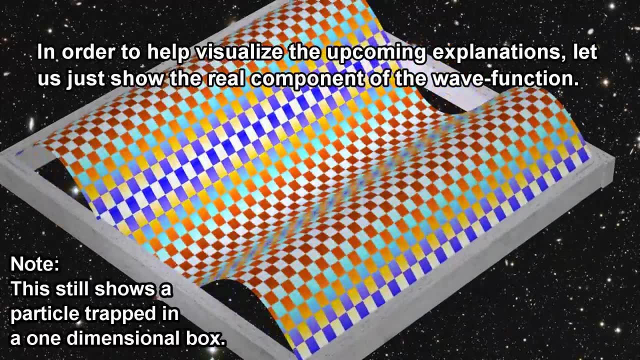 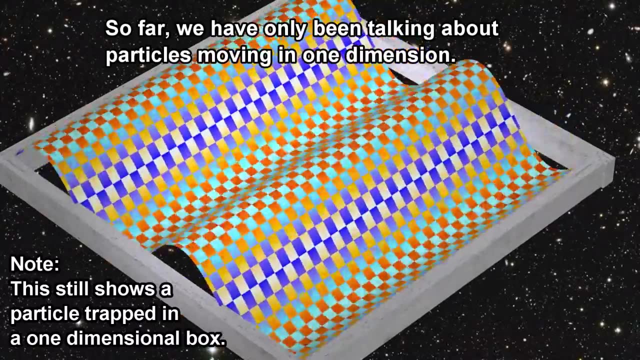 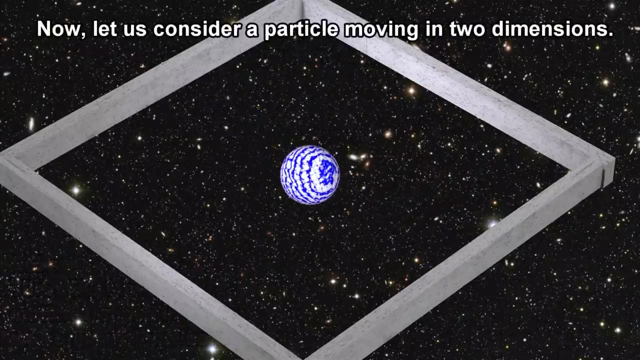 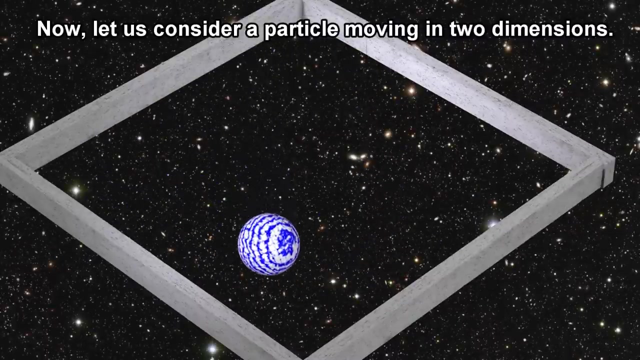 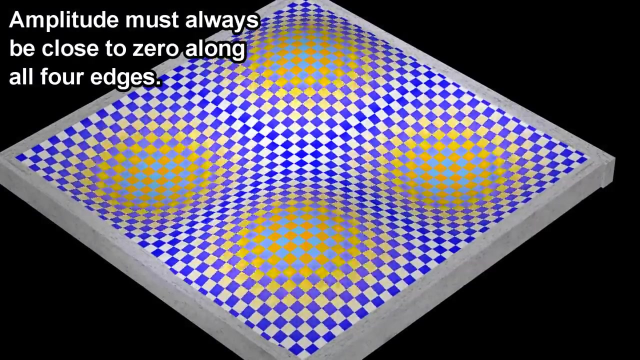 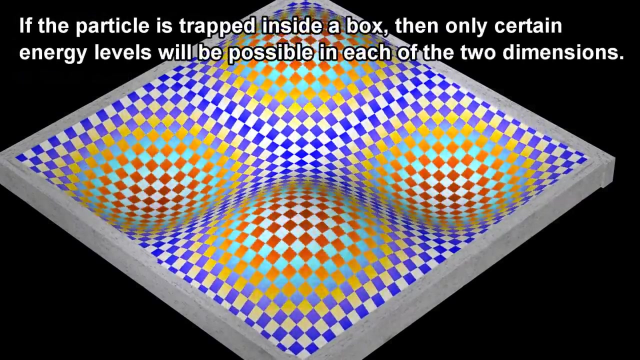 Let's drop both particles in perfect助. So far we've only been talking about particles moving in one dimension. Now let's consider a particle moving in two dimensions. If the particle is trapped inside a box, then only certain energy levels will be possible.